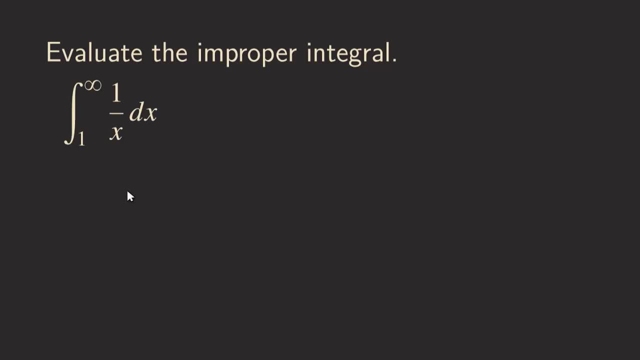 Hello everyone. it's Wilson here. Today I want to talk about how to evaluate improper integrals of type 1.. So these are the types of integrals that has an infinite interval. So, as you can see here for this example, here we have 1 to infinity, And so the way that we are going to start is that we 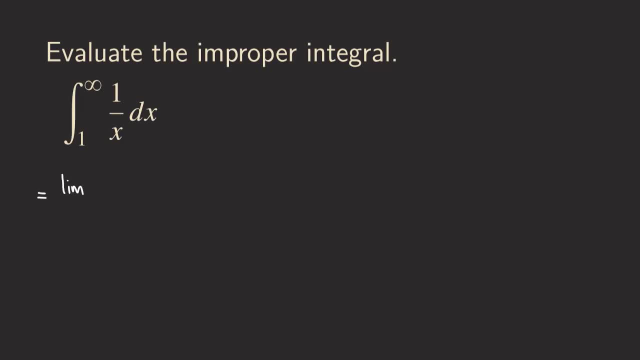 are going to start by using the definition. So we write this improper integral as a limit of a definite integral. So we have the definite integral from 1 to b, where this b is approaching infinity. Okay, so we are going to get the same integrand here: 1 over x. Okay, so first, 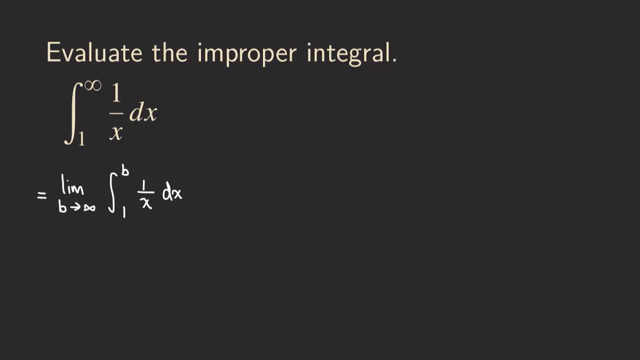 we are going to evaluate the definite integral And then after that we take the limit. And so now we are going to just write down the limit here And then, integrating 1 over x, we are going to get a Ln of absolute value of dx. That's the int derivative of 1 over x. And then we evaluate. 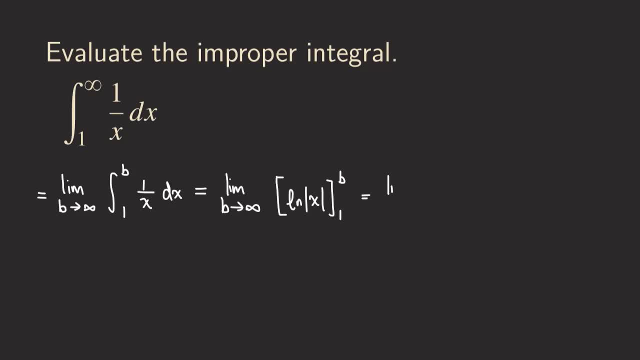 from 1 to b, And then, so now, using the fundamental theorem of calculus, we can plug the b into the x, plug the 1 into the x and then subtract them, So we have Ln of absolute value of b minus Ln of absolute value of 1.. And then, so just to see that Ln of 1 actually, 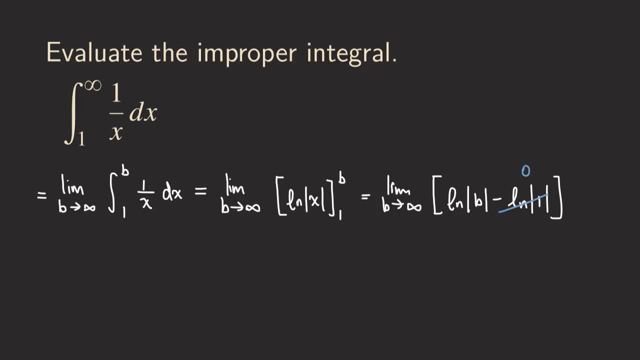 is zero. So we only need to worry about finding the limit of Ln of b, And so we have the limit as b goes to infinity, and then Ln of absolute value of b, And so when b is approaching infinity, then Ln of b is also approaching infinity. So our answer is infinity. And so what does? 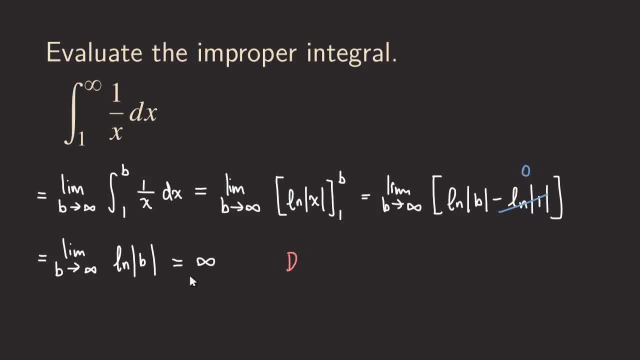 that mean. That means this improper integral is divergent. Okay, here's another problem: bytes. this time we have the lower limit as leg of infinity and the upper limit is zero, so we are still going to use the definition to write that as the limit. And so we have a approach: the leg of 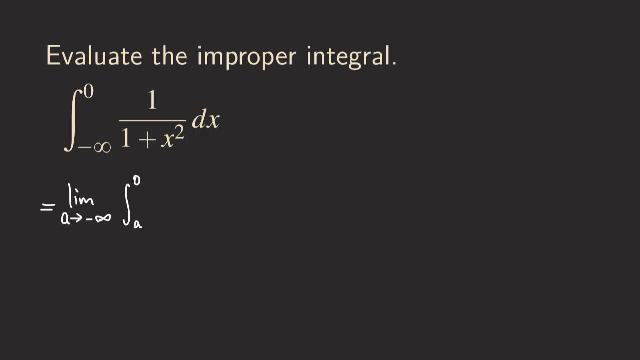 infinity. the integral is going from A to zero, And then integrand is the same, so one over one plus x square, dx. And so what happens is that we are going to integrate- Integrating this one over one plus x square, we get dx, And we're not going to multiply the integral from infinity to infinity. 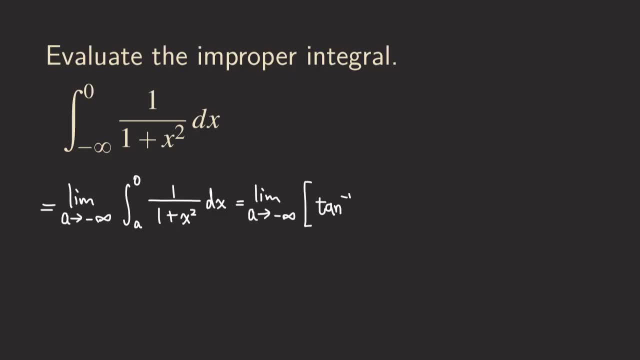 because, in other words, everything should be innocent to us. combined with 1, x squared and ง to one times aahoop. So theranean lounger is arctangent. So tangent inverse of x, Evaluate from a to 0.. And then, so now just plug in. 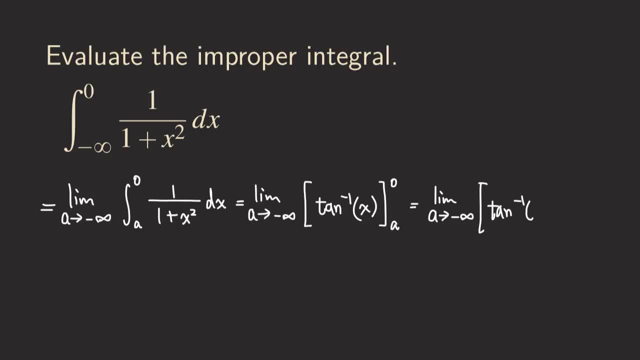 Okay, so we are going to get tangent inverse of 0 minus tangent inverse of a, And then see, the tangent inverse of 0 is 0. So we don't need to worry about this one. All we need to worry about is just the negative tangent inverse of a, And then we're taking the limit as a approaches. 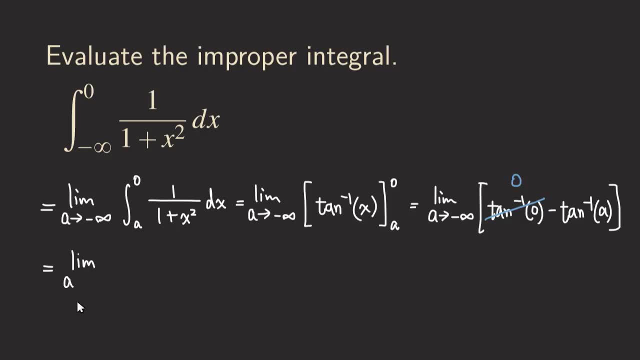 negative infinity, So negative tangent inverse of a. And so now the question is: what is this limit equal to? It would actually be a good idea to actually just just draw like a tiny sketch of the tangent inverse function, And then we can just go from there and 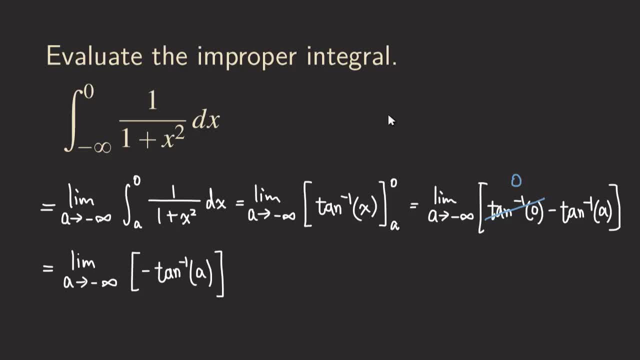 see what the limit is, And then we can just go from there and see what the limit is, And then we can just go from there and see what the limit is. Okay, so I'm going to grab it here just to make a tiny sketch of that. This is x, this is y, And then what happened is that we have 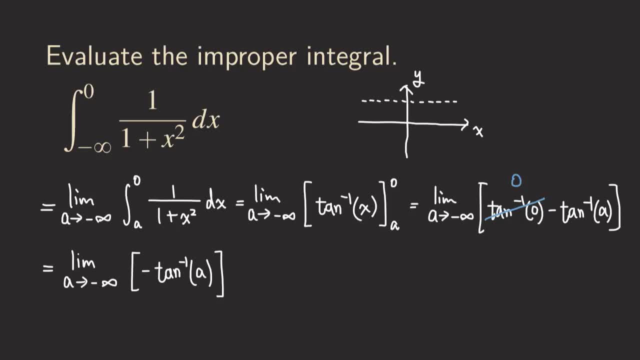 the two horizontal asymptotes for the tangent inverse function. So this is at pi over 2.. And then the other one is at negative pi over 2. And then the curve is actually: it looks like this: And then: so, when a is approaching, 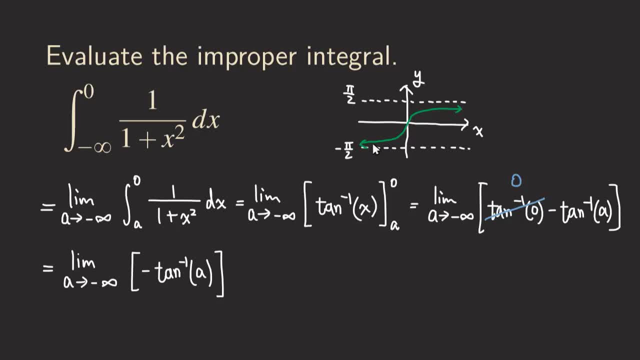 negative infinity. we are actually looking at this spot right here. So when a curve is going to negative infinity- because that's that's what a- where a is a is inside, it's being plugged into the tangent inverse. So we look at this right here And then we look at the behavior, the 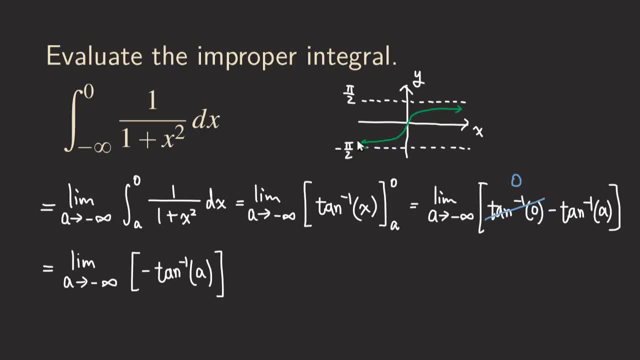 tangent inverse function, So it's approaching negative pi over 2.. And so the limit is negative pi over 2.. But then don't forget that there was a minus sign here, So we need to pay attention to that. So what happened is that we are getting 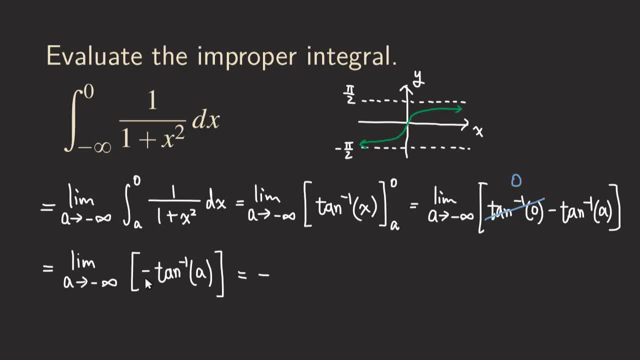 negative. that's actually coming from this negative sign here, And then also this is approaching negative: pi over 2.. So we have a pi over two, And so what do we get as the answer here? we get pi over two, And so what is the answer? This is equal to pi over two. 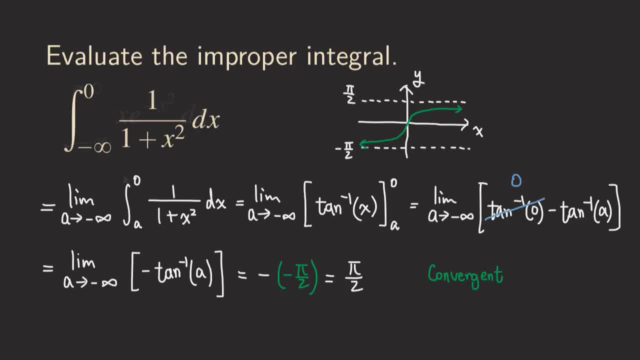 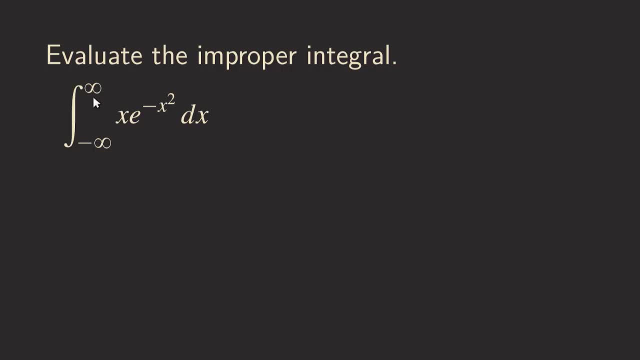 and then the improper integral is convergent. Okay, one more improper integral here this time we have: the lower limit is negative infinity and the upper limit is positive infinity. So the way that we are going to start this is to separate the integral into two, into those ones that 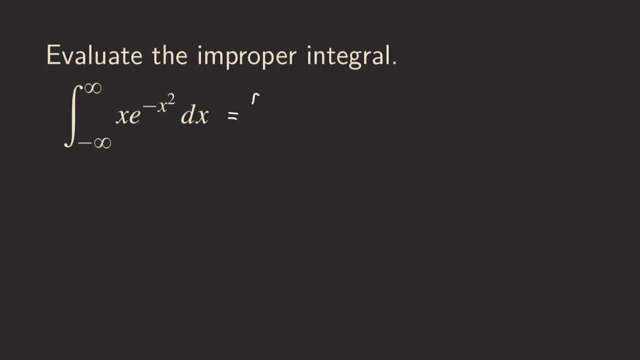 we just calculated, So we can write it as the integral from negative infinity, and then x, e to the negative x square as the integrand. And then what happened is that we need to choose a convenient point for us, and convenient value that we can choose would be zero, And so now we have the two. 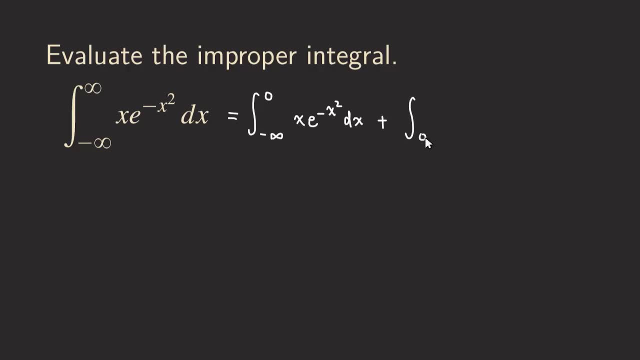 integrals. And so now for the second, and the lower limit would be zero, and then the upper limit would be the positive infinity. So we have the infinity here, and then x, e to the negative x square, and then the x. Okay, 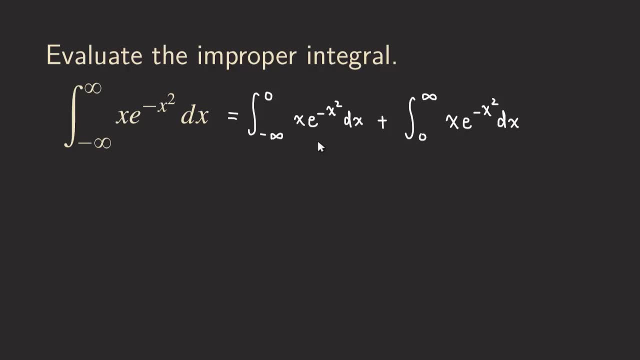 so because we need to compute both. then what happened is that we would need to find the antiderivative first. So it would be a good idea because it will work for both integrals when we find the antiderivative. So we just need to make sure that if they both converge, then our original 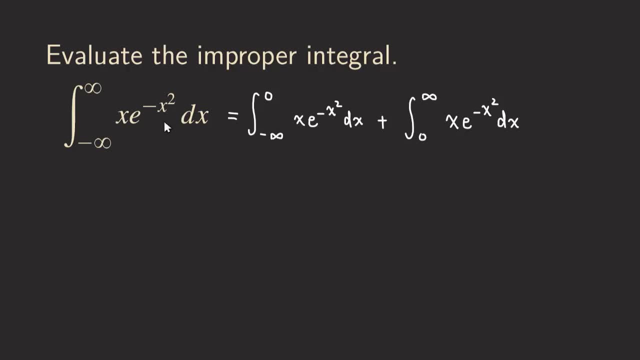 integral will converge, But if we don't, we're going to end up with a negative integral, So one of them diverges, then this original integral will also diverge. Okay, so we are going to just find the antiderivative first, And that would be just to. let's do that here. So integrating 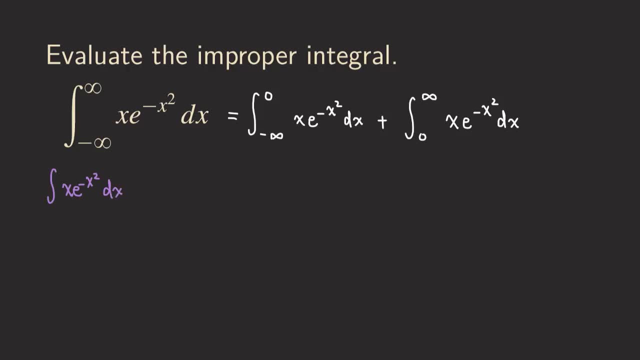 x e to the negative x square dx. And so what happened is that we are going to do a use up so we can let u be negative x square and then the? u is going to be negative two x dx, And then you get: there was an x here, there was a dx here, there was x here, dx here. so we can isolate the. 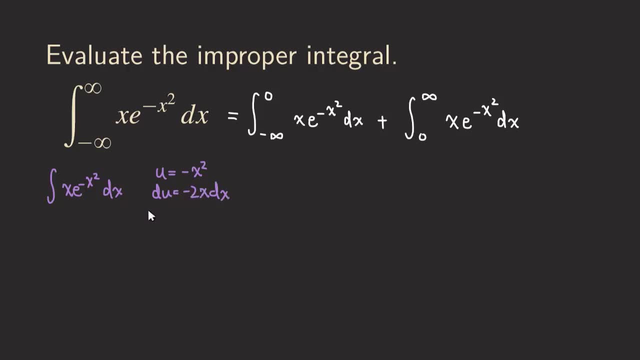 x dx, and then we move the negative two to the other side of the equation. So we are going to get negative one over two. du is equal to x times dx, And then. so what we get here? we are going to get negative one over two, and then the integral, and then this is x dx. right, it's replaced by. 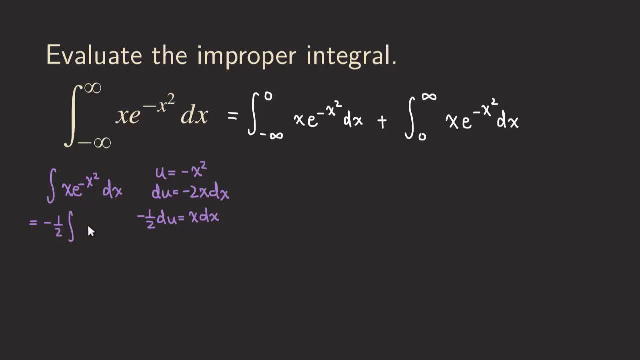 negative one half, and then du. So there is the du here, and then we have the integrand s e to the no, just e to the u, which is just like the one over two e to the u, and then put back the. 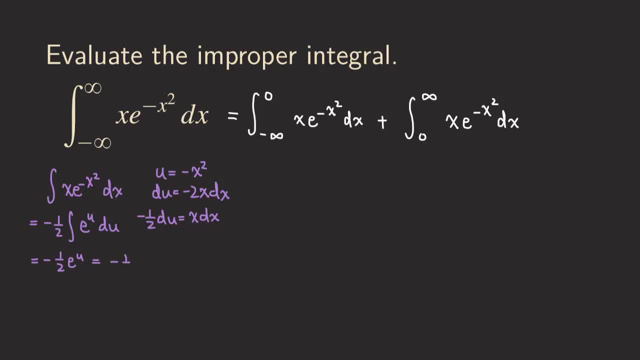 negative x square into the u, So we get either one over two e to the negative x square. And then there was a plus here, but we are not going to write it down for now because we are going to have actually a definite integral. Now let's compute this one. So computing this one. 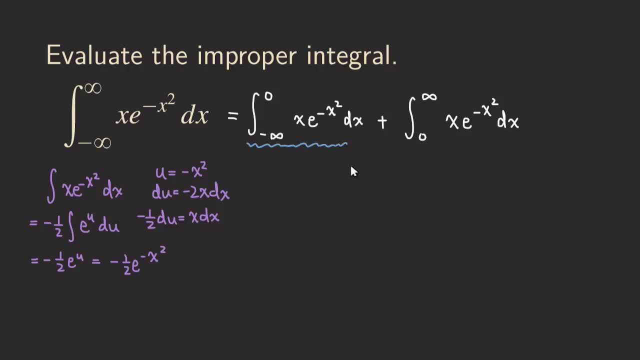 actually let me just use, let me just highlight this, I'm going to do it in the different colors- So this integral, like the infinity to zero, x, e, to the negative x, square dx. So what happens is that we are going to just write it as the limit of a. 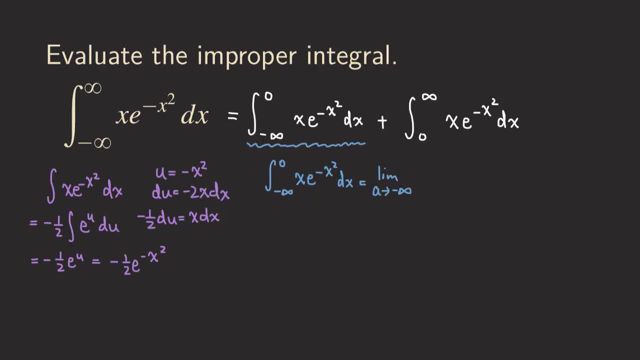 definite integral here. So we have a approaching late infinity, just like the second example. So we have going from A to zero, and then x, e to the negative, x square dx- Okay, and then we already have found the antiderivative, Okay, so we are just going to. 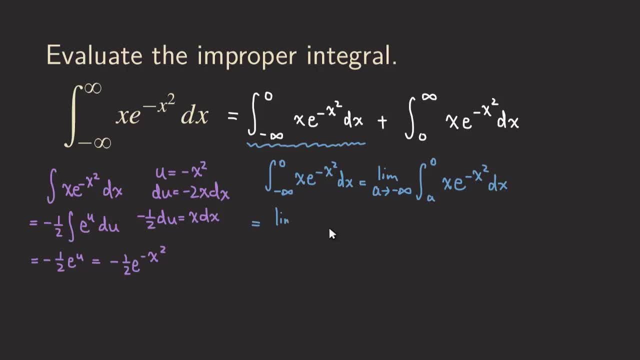 continue. So we have the limit as a approaching negative infinity, and then nt derivative is negative one over two, e to the negative x square, and then you value it from a to zero. plug in the plug in the zero in here. So we get negative one over two, e to the negative zero. 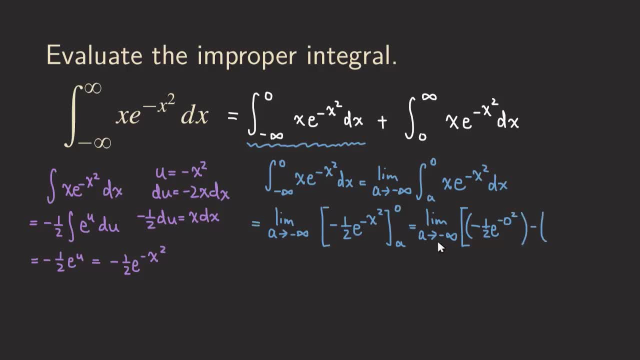 square and then minus. now plug that a in here, So we get negative one over two. e to the negative, a square. Okay, so just continue from here. we have the limit as a goes to infinity. Now what do we get from here? we get negative one over two because e to the zero is one, so we get negative. 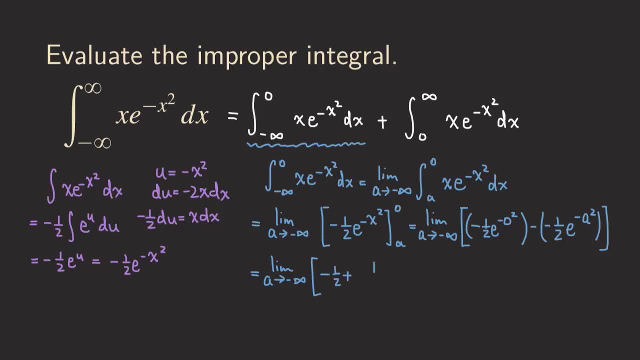 one over two and then plus one over a. why do we get a plus here? because there was minus, minus, right. so we get a plus, and then the two is in the denominator. there was also e to the while there was a negative. 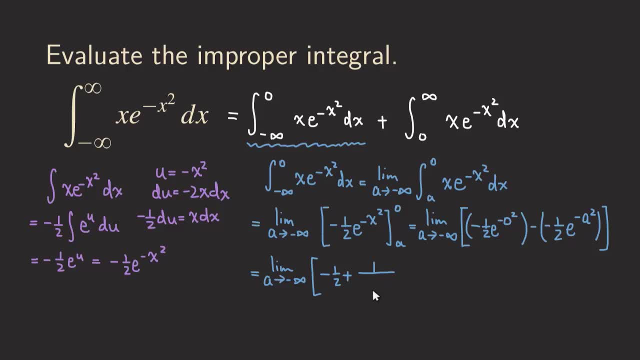 exponent here, So also in the denominator. so we are going to get two and then e, a square. So now see that we have a score as the exponent of the e. So when a goes to negative infinity, we score it. we get positive infinity. So the denominator is approaching positive infinity. So 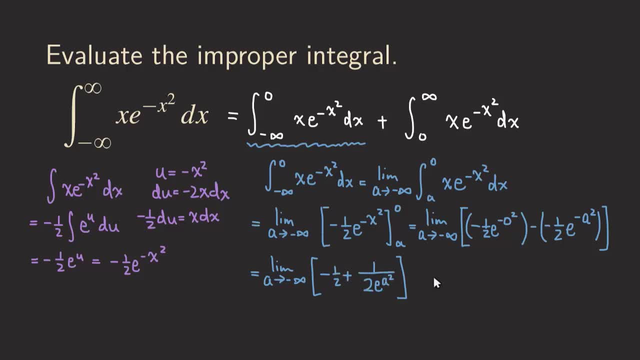 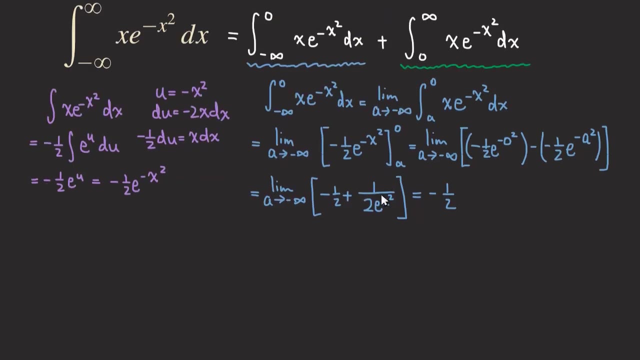 the whole thing is actually approaching zero. So we have the answer as negative, one over two. So this integral, this first one right here, is convergent. Okay, so we say that that one is convergent, But now we still need to look at the other one, right? So let's do the the other one. So we're doing the second one. 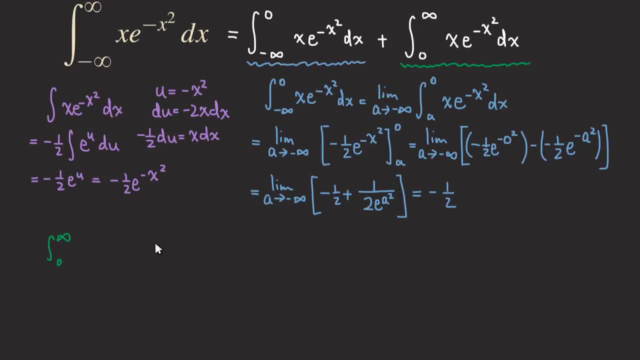 let's do it right here. So we get the integral from zero to infinity and then same integrand, And that's the limit. as B approaches infinity, we're placing the infinity with a, B, and then we have the zero. at the bottom, we have x, e to the negative x square. 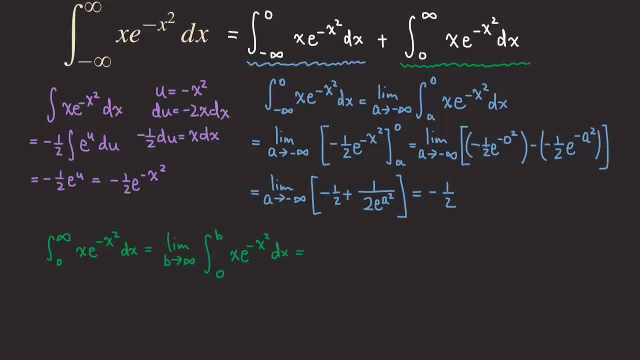 dx And then. so now what happens is that we are going to just start plugging in the nt derivative in here. Well, actually we are actually just replacing the integral by the nt derivative, not plugging in, and then going from what? going from zero to be continuing from there. So be going. 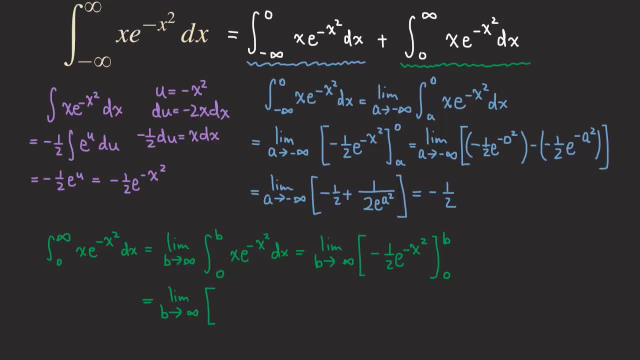 to infinity. then we have now plug the B in here, plug the zero in here, subtract, And so just write it like what we had here, as a fraction, so so that there was no negative exponent, which will make it easier for us to evaluate the limit. Okay, so let's. 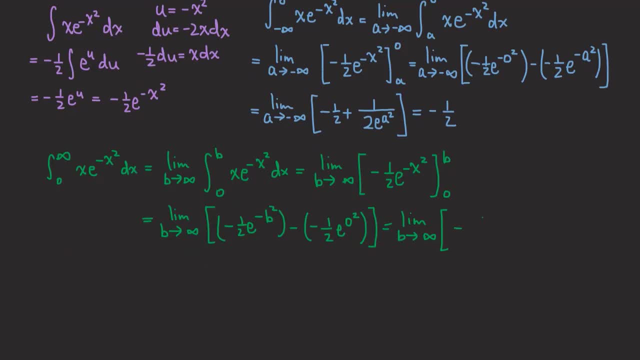 continue from there. So we are going to get negative one over and then two, and then e to the B squared, Okay, and then plus. then again there was a minus, minus here. so we get a plus, and then we have positive one over two. And so just like before, because there was a B score here, 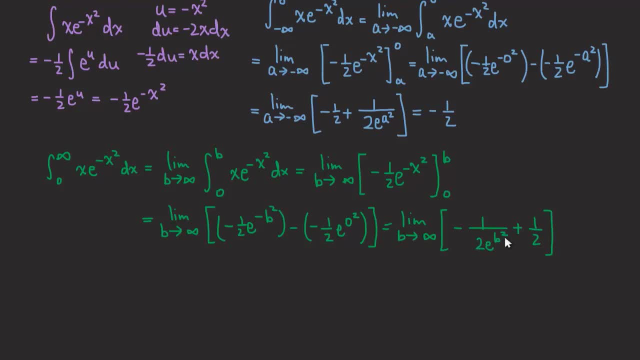 that is the exponent of the E. So when B goes to infinity, this denominator is approaching infinity, So this whole fraction is approaching zero. So we only need to worry about this one half here. Well, actually the answer will just be one. So the second integral is also going to be a plus.